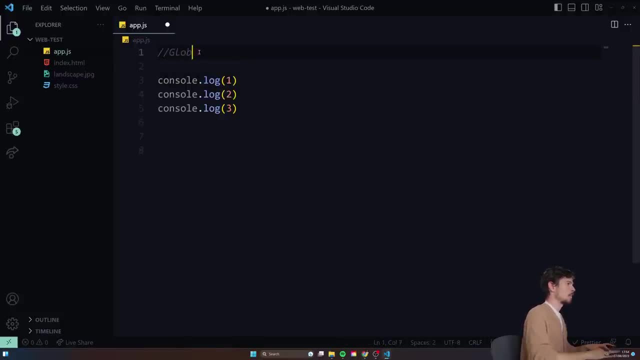 running up here is called the global execution context, All right. and there is one more context to be aware of is the function execution context. So if I make a function here called like logger and I'll just say console log two and three down here, All right. so if I 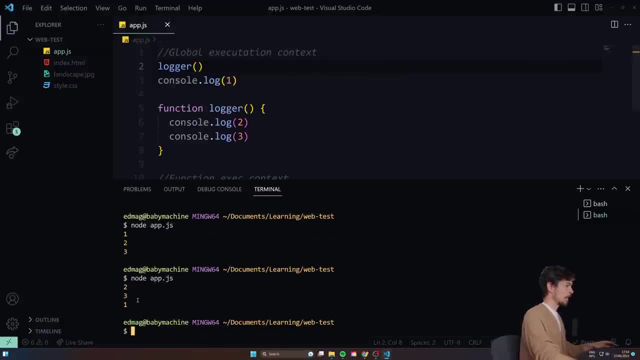 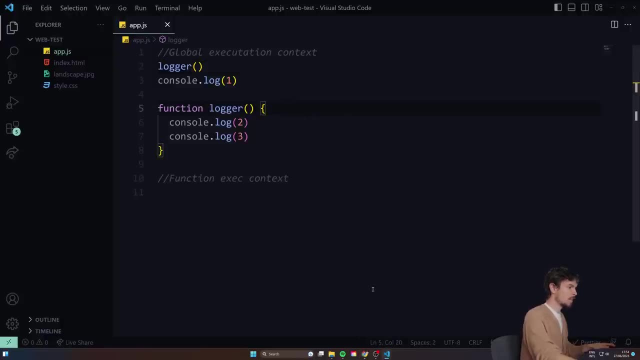 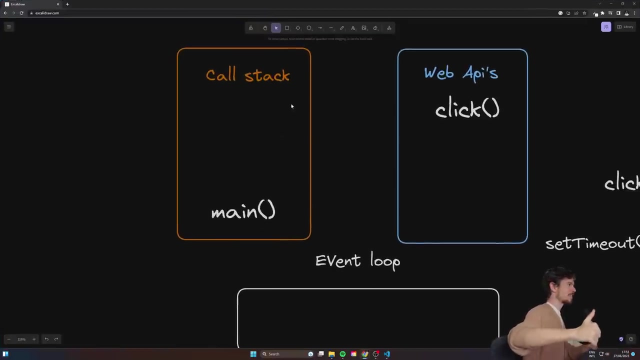 run, logger up here and run this. we are going to get two, three and one. Why is that? Well, there's a concept called call stack And I'll show you this. Thank you so much, TOGG, by the way, for this Excel to draw thingy that I saw that you're using It's. 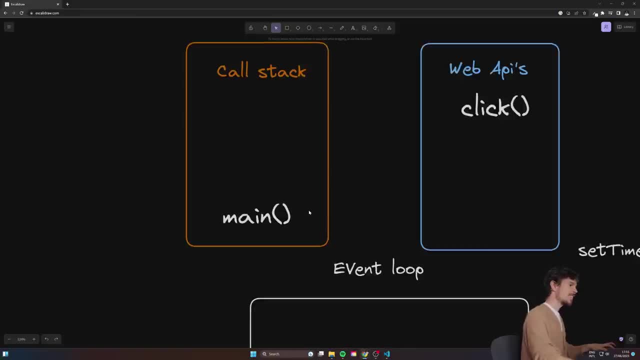 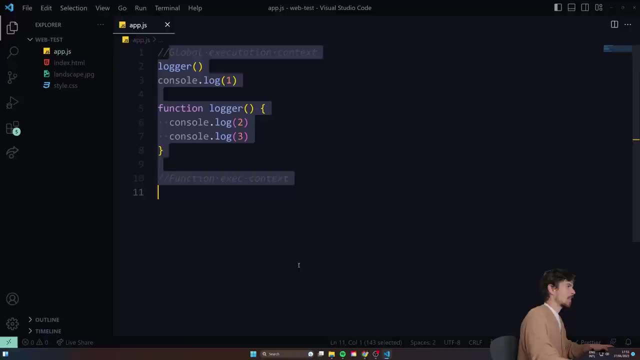 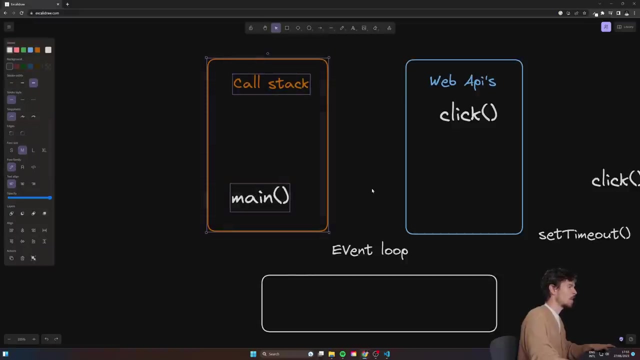 fantastic. Goddamn The blend, Just then. Sorry, I love that song Anyway. So what happens is the environment that we're running our code is essentially our global execution context, So that gets added to this thing called the call stack right here, And the call stack is a way to keep. 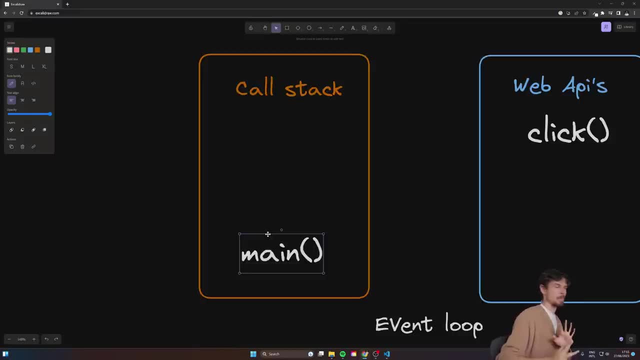 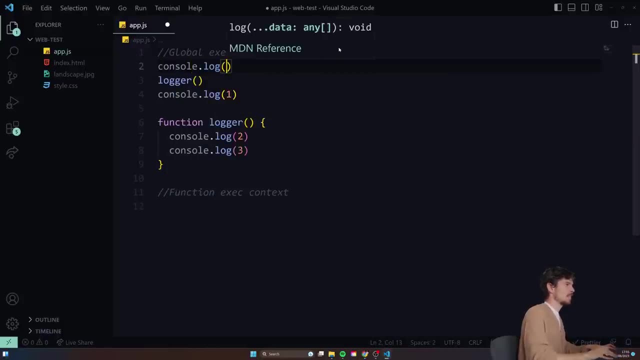 track of what code we're running at what time. All right, it's just a way for JavaScript to know what the hell is going on. So if I have something like a console log message here, of course that's going to run first. 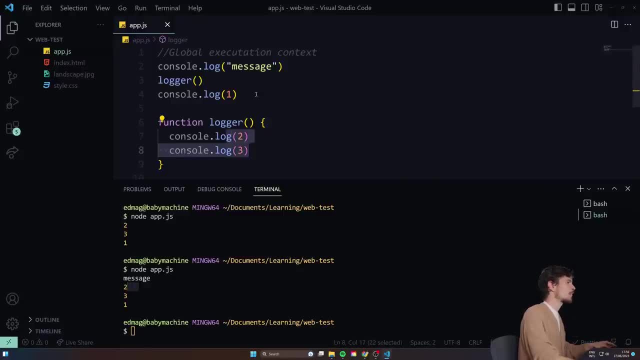 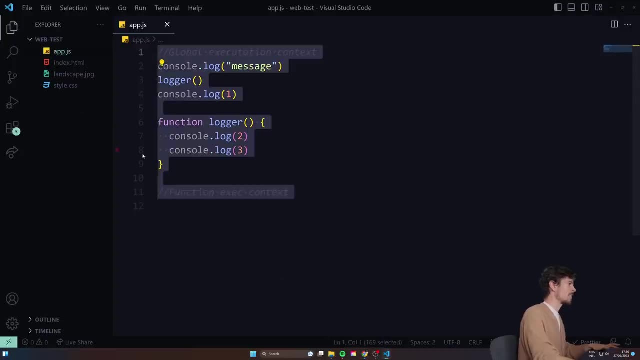 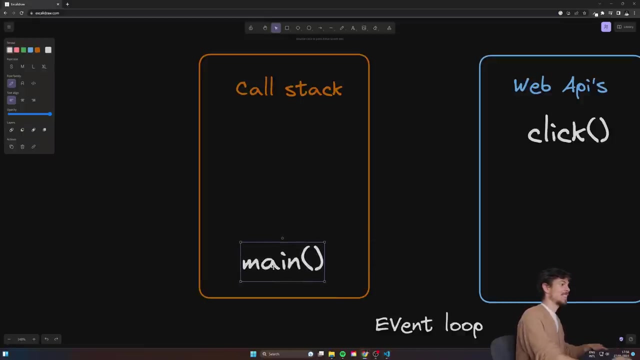 right. So if I run this, we get message, but then we get two and three. We're not getting console log one here. So why is that? Well, our main here again is our main execution context That gets added to this call stack, And the way the call stack works is the things get stacked. 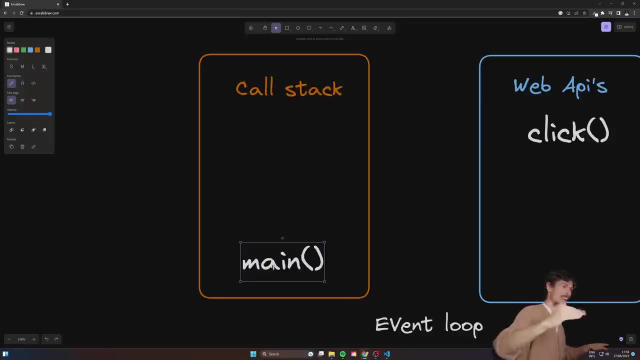 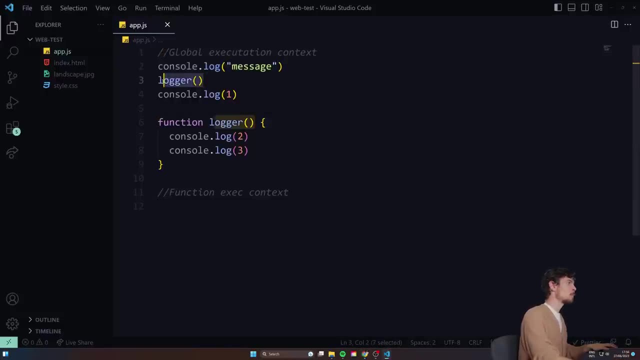 on top of it, right, And the things that are on top of it get executed And once they finish moving, it's going to be moved. So in this case we run console log message here, but then we run into our logger here, right, Which has its own execution context. So what we do when we invoke 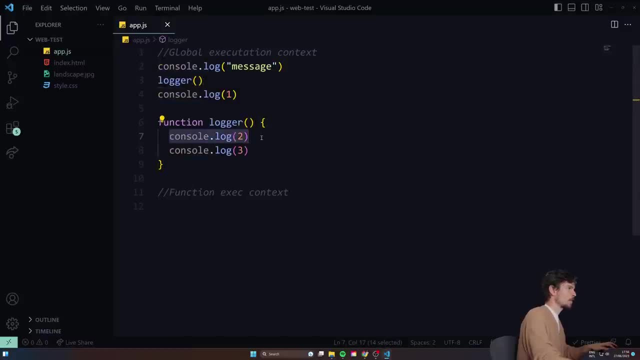 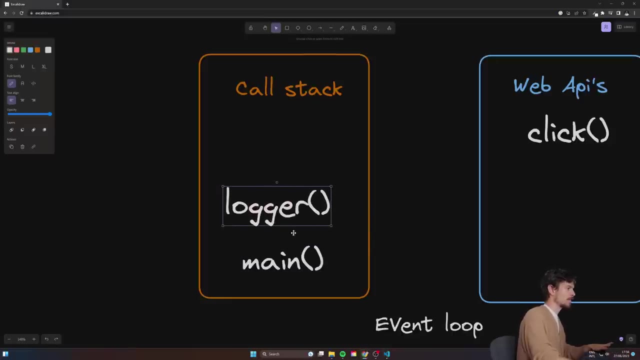 a function, we start running the code inside that function. So we run two and three So that essentially gets added here to the top of the call stack. So our main thread here, our main execution context, is going to be stopped, All right. So nothing is going to be stopped, All right So. 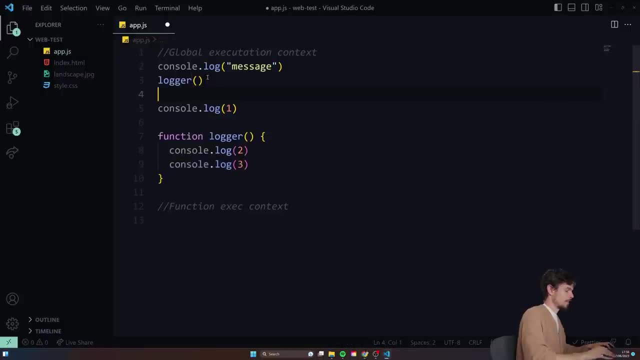 nothing is going to be stopped. All right. So nothing is going to be stopped, All right. So everything here below the logger. so I'll put a stop. Come on, There we go, All right. So once the logger starts running here, everything below it will be stopped until our logger is finished. 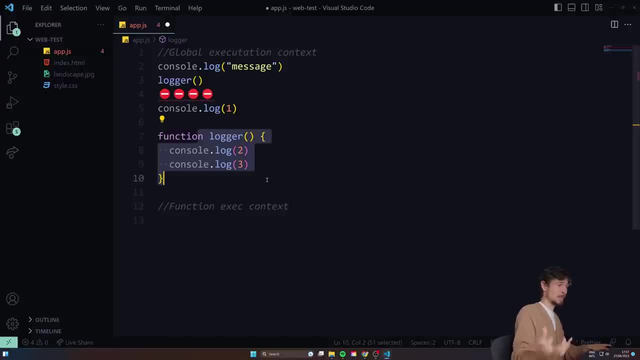 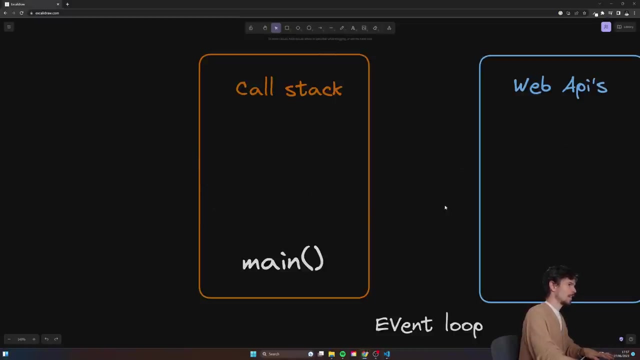 returning Now, whether that's a value that it's returning or it returns nothing, just void. it needs to run fully before we can continue down in this main context. All right, So once logger finishes, it gets popped off the call stack here And then we can. 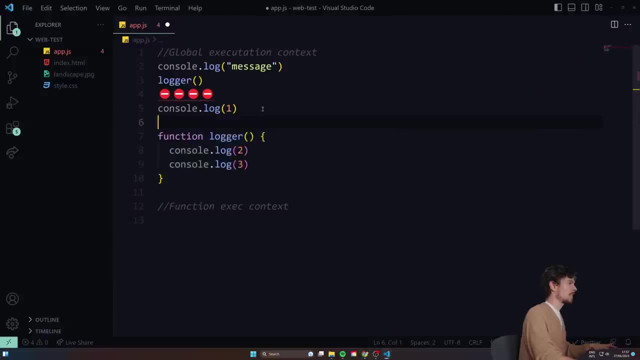 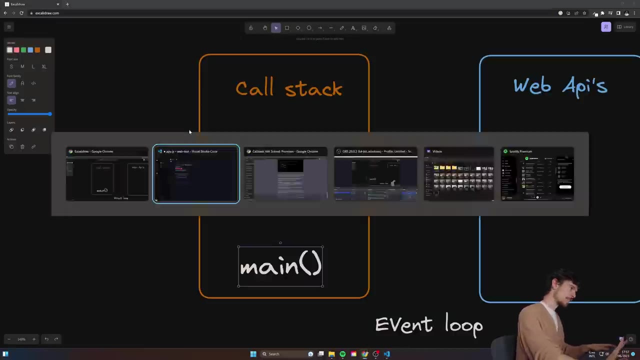 keep, continue to run our main. So our main is going to keep running console log one, And once that's done, boom, our call stack is empty. All right, So that's the idea behind it. Now you can do more complex examples If you want. you might have logger there, but you might also run another. 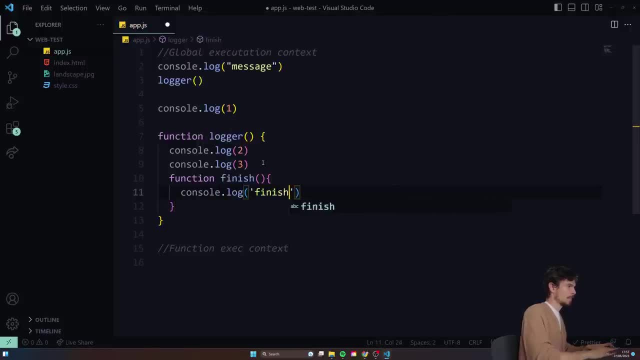 one, And then I can run console log finished, like that, And then I can run this, maybe here, All right. So how is this going to run now? Stay with me, We're going to get to prophecies, I swear So again. we're going to run our main right. So it's going to run message. Then we get. 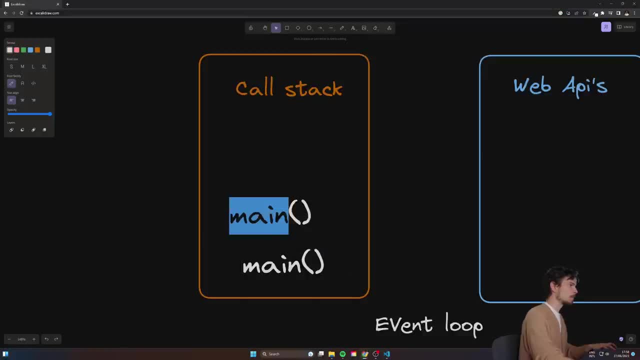 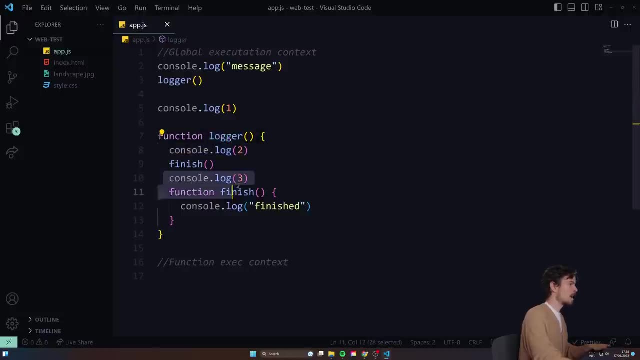 to our logger. So we're going to go into our logger. That's going to start executing here. All right, We run console log two, but then we pop and we don't run console log three anymore because we're invoking another function here. 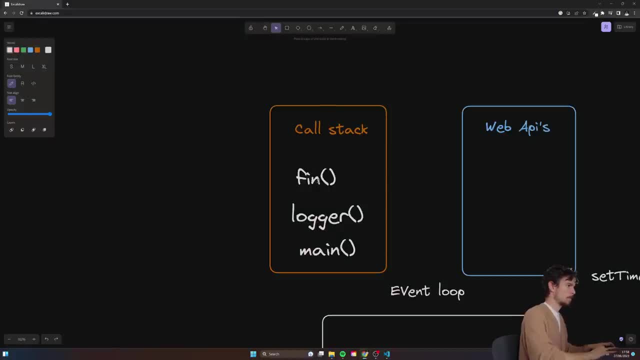 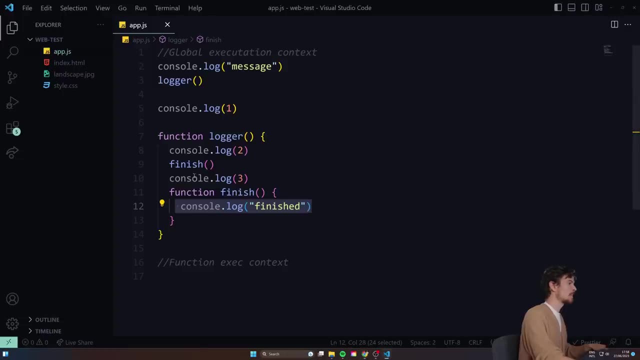 So finish gets added to the top And then finish is going to run console log. That's going to be finished, So it's going to get popped off. Then we can continue with logger. So we're going to run three. That's going to be popped off And then we can continue with the rest of our global. 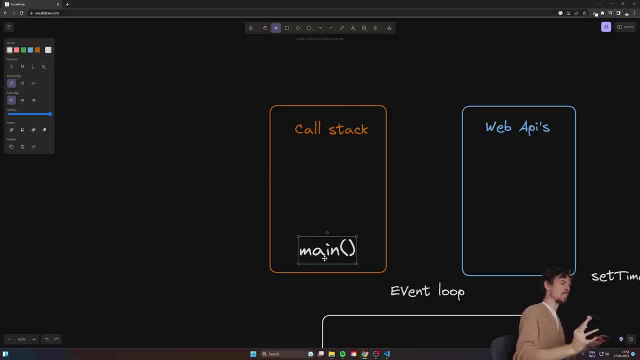 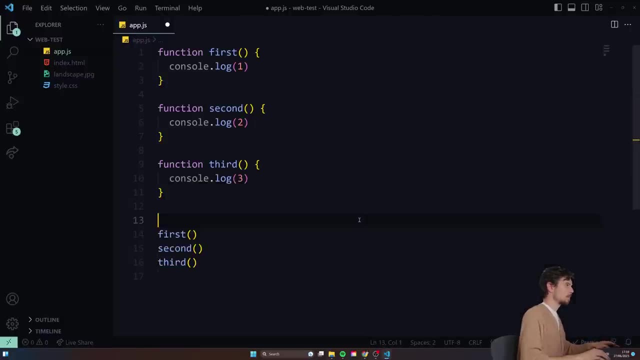 execution context. All right, So that's the idea behind the call stack. It's a way for JavaScript to know how to run your code. Okay, So here's another example where we have just three functions that run console log: one, two and three, and then one, two and three. So if I run this, 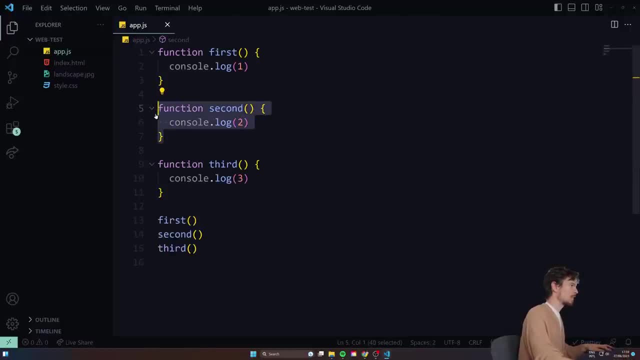 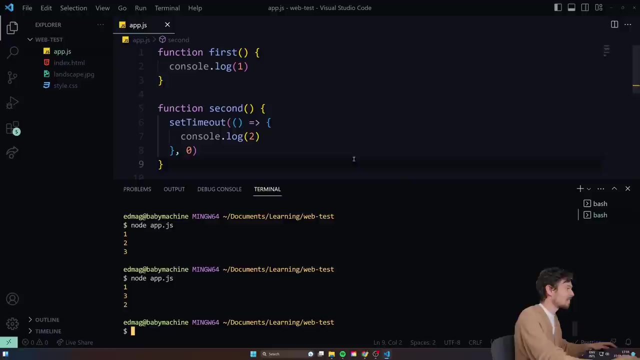 yeah, just what you expect. However, I'm going to take the second function and I'm going to replace it with a set timeout. Now, be aware that the set timeout here is set to zero, So technically it should still run instantly right? No, it doesn't. We get one. three: 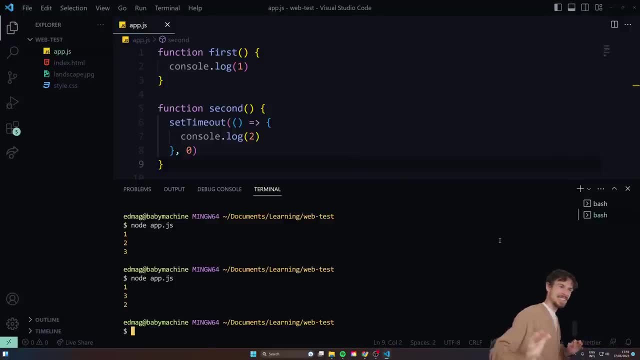 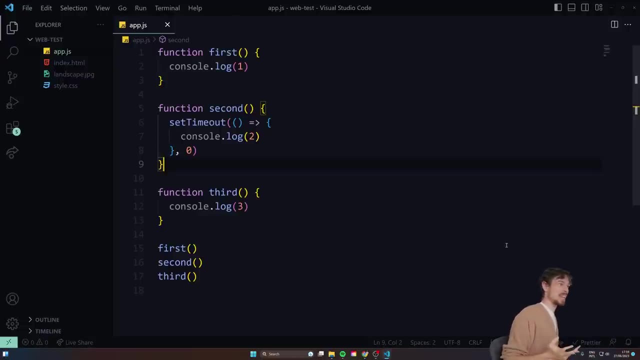 two: Why, Why, Ed? Why Didn't you say everything is running synchronously in JavaScript, Single threaded? That's what you kept saying. That's still correct, Even though this does look like it's running asynchronously technically. it's not. What we're doing is we're offloading. 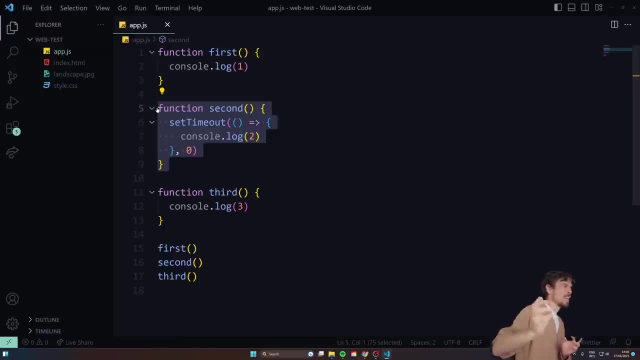 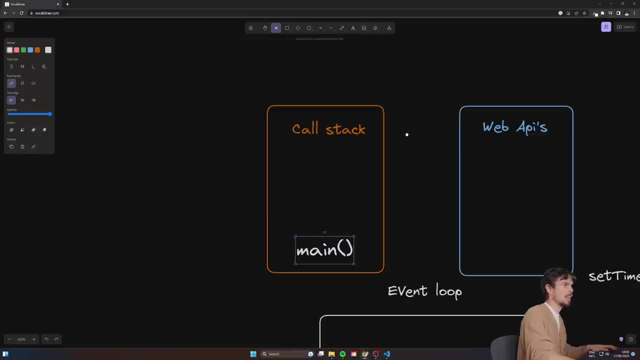 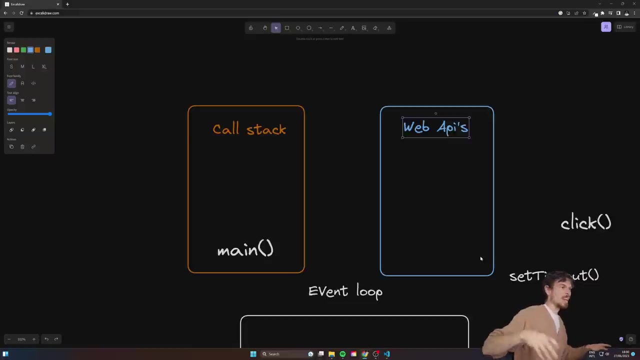 the set timeout, All right. So besides the call stack, what else we have here? Let me pull up the graph. We have web APIs like click, set, timeout, set interval, scroll. Imagine you have like an on click listener. If that would be added to the 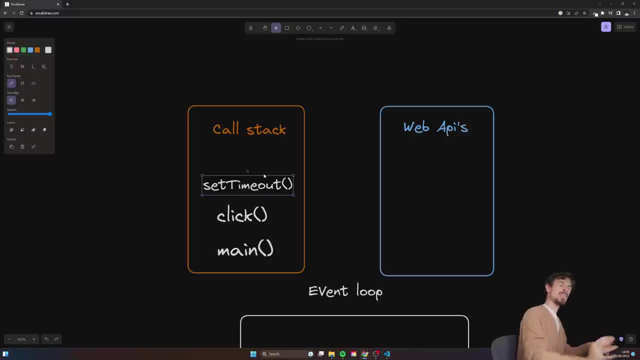 call stack or maybe a large set timeout here. we wouldn't want to block the rest of our code from running. right, Then our websites become unresponsive. Like well, if I have, like a button that signs the user up, does that mean the rest of my code's website couldn't run? 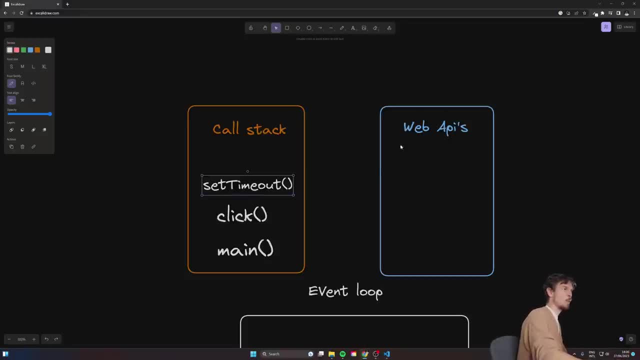 So what we're doing essentially is we're taking these things, these web APIs, and offloading it to the browser to run in the background. So let's say, we have a set timeout of 5,000 seconds here. Can I not modify this? Okay, 5,000 seconds. What we're doing is the call stack is going. 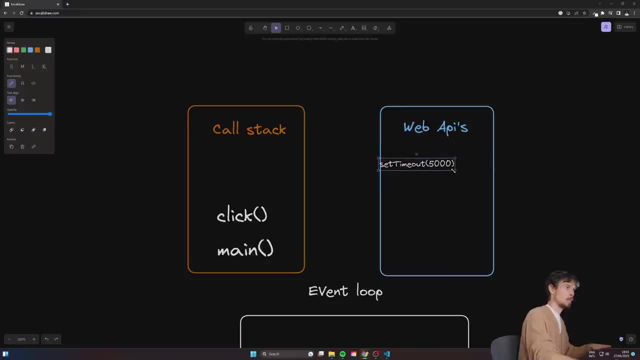 to pass it down here into the browser's web APIs, And the browser is going to start running that in the background for you: Tick tock, tick, tock, tick, tock. Time's up, motherfucker. And when the time's up, there's this event loop here And the event loop's job is to start queuing. 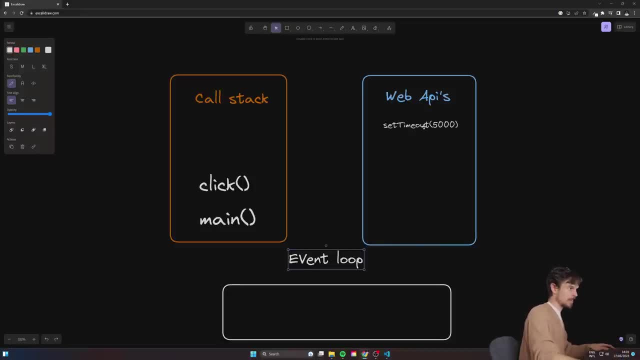 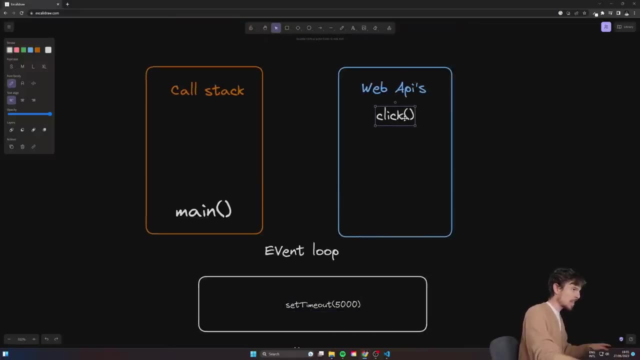 stuff up to be added back to the call stack. So once this is done, five seconds is run, it gets added to this callback queue. All right, You might have active things running here as well, like a click listener that maybe when you click it's going to like: remove a to do. 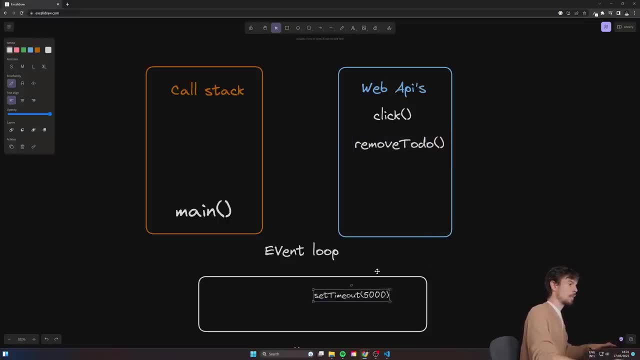 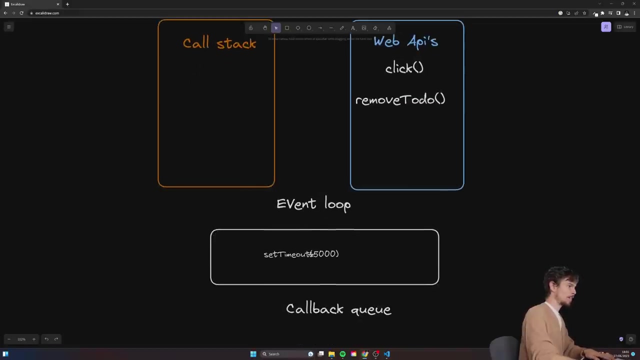 Like that. All right. So what happens here is: let's see, this is running here right Five seconds, And then it gets added to the event loop here And then, once our whole call stack is finished- so there's nothing else running, the event loop's job is to start pushing things from the callback. 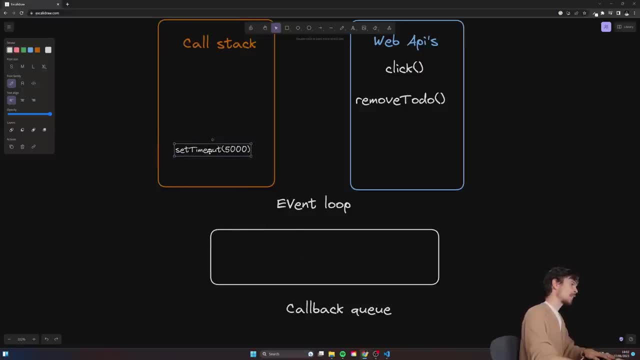 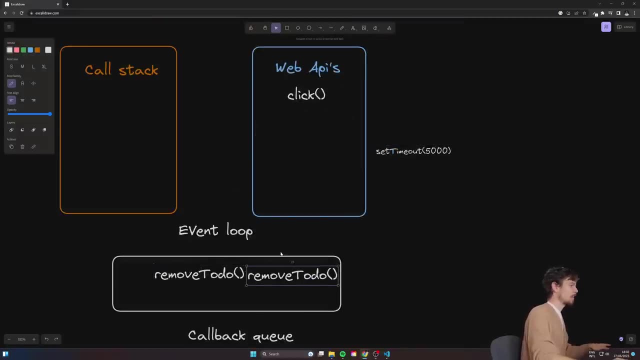 queue back to the call stack And then, once that's finished running, poof, it's going to remove it. All right And same. like: if you click on this button, it's going to start putting: let's say you click three times, Well, it's going to add three different things, three different separate. 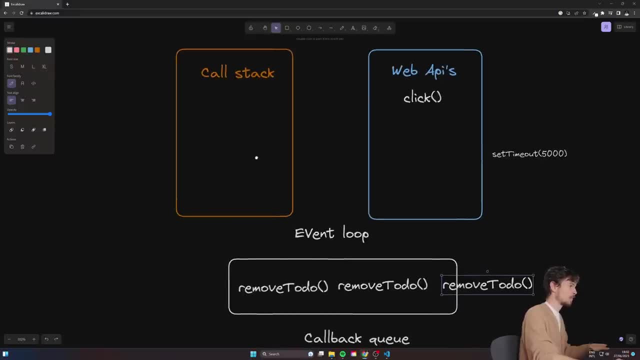 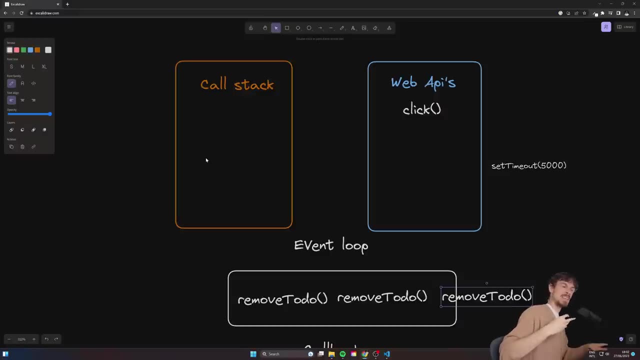 functions here to be ran as soon as the call stack is finished running. That's why you might have like a slow website running. You might have some weird funky code, maybe like you messed up a loop that's running for too long and you click on a button and it's like nothing's happening. 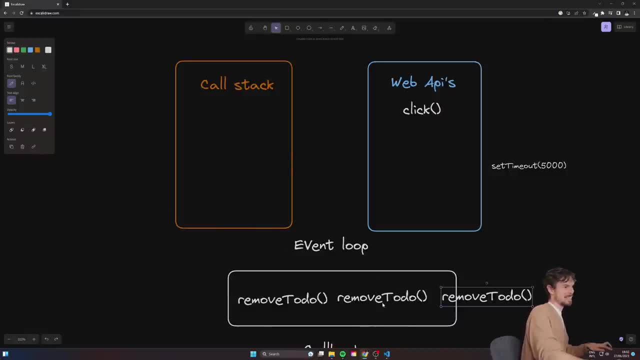 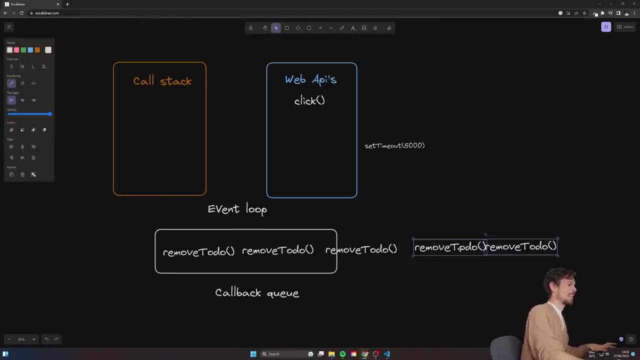 And then all of a sudden you get poof, poof, poof. It's because your callback queue has like 10 different remove to do's queued up And then, once the call stack actually finished that large loop, it's just going to push everything all of a sudden on top here like that. Oops, sorry, It should be. 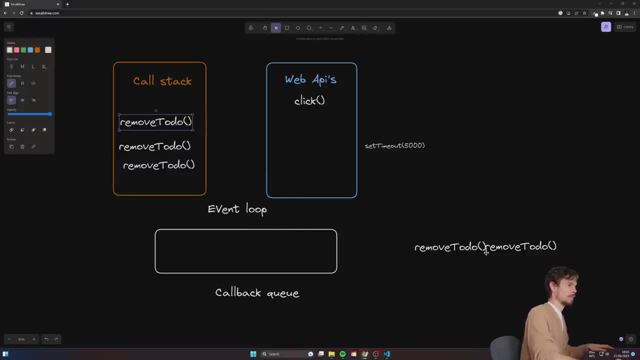 like one on top of each other. That's how the call stack works: First in, first out, I think it's called. And then boom, boom, boom boom. They would start disappearing, like that. Okay, So that's kind. 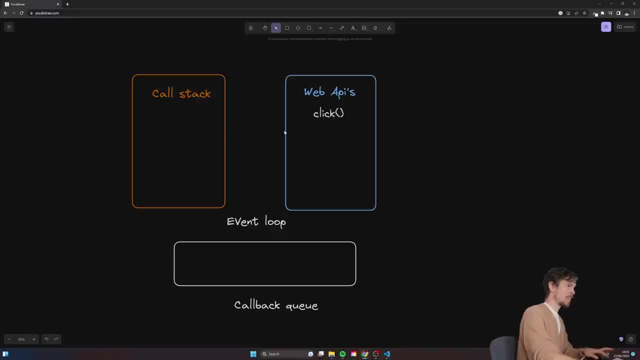 of the mechanic behind it. It's this call stack, together with the browser's APIs, that gives you the ability to run stuff in the background. but it still runs synchronously because essentially, just like queues everything up here to run synchronously anyway, at the end it just stops. 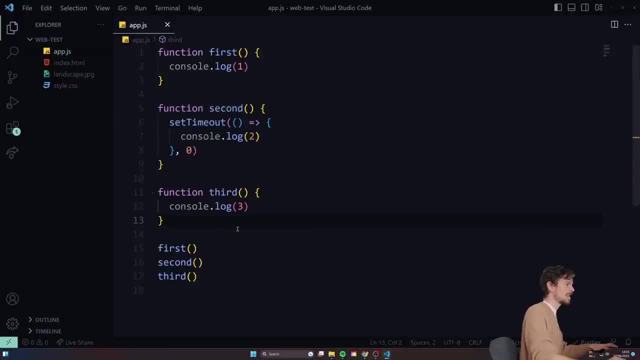 it from blocking the main thread. So how can we take this idea? Because it's unclear now that- oh damn, you know, the second one has actually come last, right, There's no clear way of seeing that. So that's where the concept of callbacks came in. So I'll just, I'll just remove this. 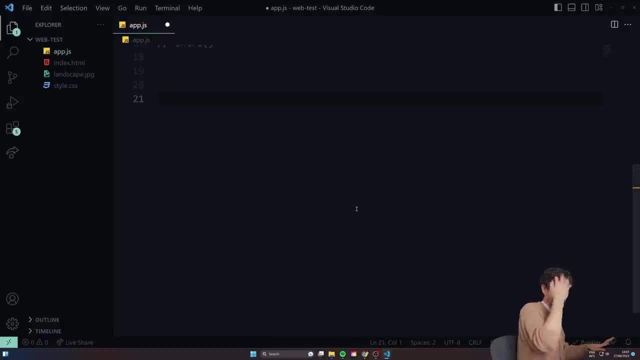 example. for now, All right, All right. So what's the callback? Well, essentially it's a function, that's a parameter. So you can have a function let's see like a logger here. um, that that's, let's just say that takes in a message, right? 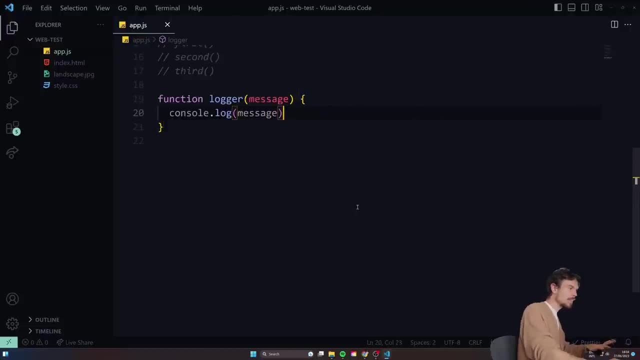 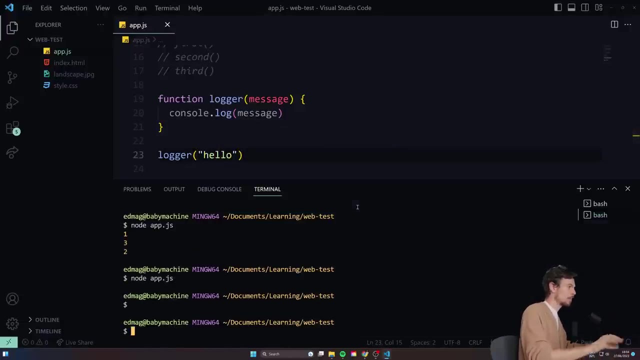 Console log message. All right, So this is just a normal parameter, So I can pass in maybe a string: Hello, All right, Normal function. Why did that not work? Hello, There we go, I work now. Okay, cool. 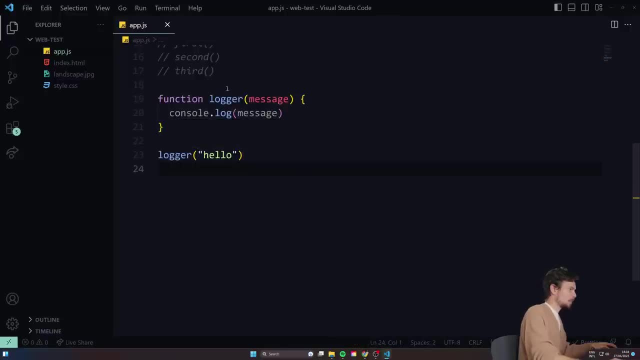 Um, all right, So normal function. However, if I take this message and not make it the string, rather than making it string, I pass in a function, So I'll call it message and I'll just make a message function here. That's gonna say console log. Hello, there again. 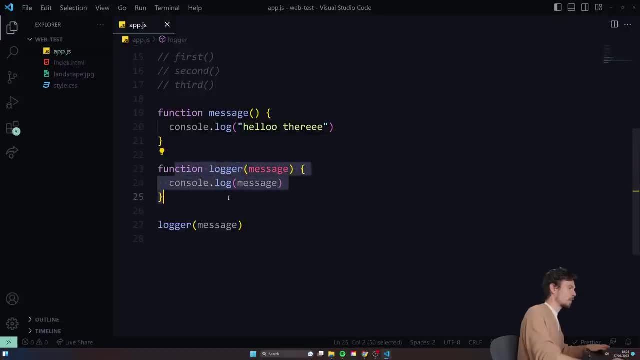 Essentially, this became a higher order function now, and the higher order function is just a function that takes in another function in as a parameter. All right, And this is our callback here, this message now. All right, So if we run this, we get hello there, but how does this apply up here? Well, 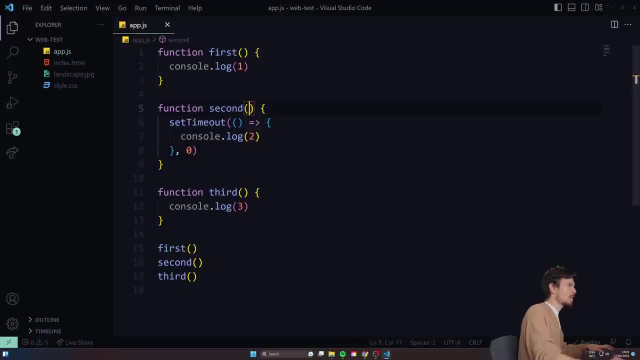 rather than doing our code like this, what we can do is in the second, we can pass in a callback right Here, callback, And I can run the callback right here, All right, So rather than invoking the third function, we can pass it in as a callback, like that. So now this third is going to be added in. 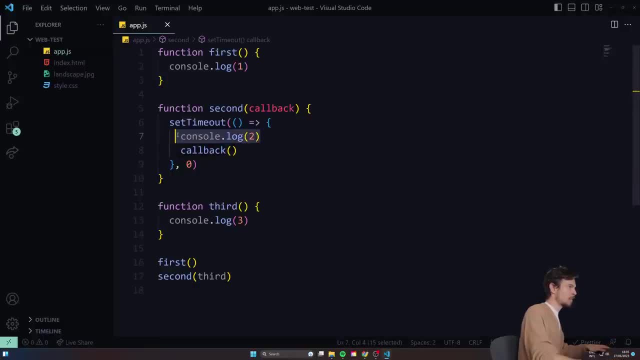 as a parameter and it's going to run after console log two here. So if we run this we get one, two and three kind of the behavior that we want to see. Problem with this approach is that it can get really messy and hard to read. I don't know about you, but I'm already having a hard. 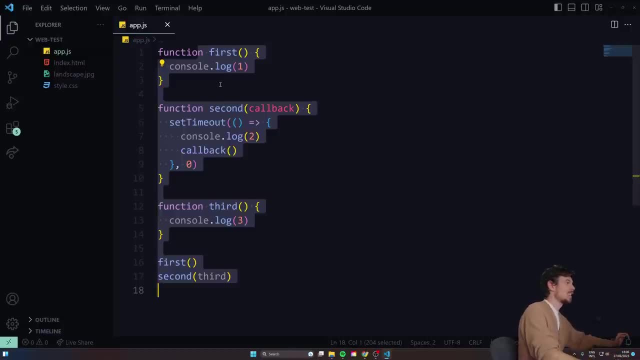 time. I'm getting three different types of migraines going on up here looking at this code. But let me show you another example. What if we get some data back and then we want to do something with it, and then we want to fetch some more data, and then some more data and some more? 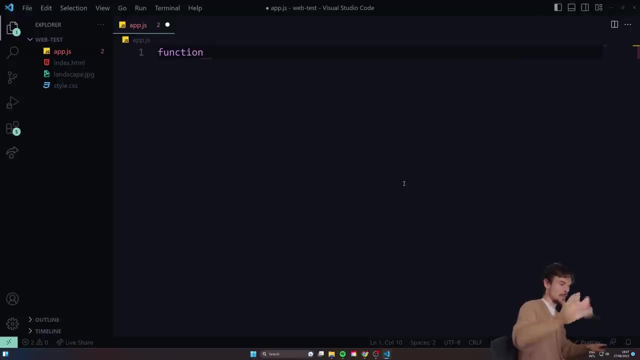 data right, Or we want to fetch some data, modify it and save it and push it somewhere else And then, based on that result, we want to display maybe a message on the screen So you can make a callback. Hell, all right. This is kind of the problem that most people ran into. 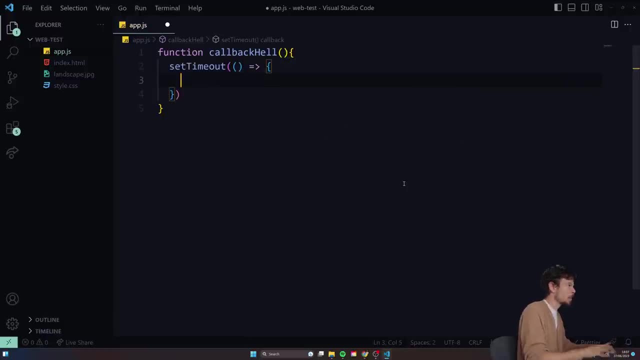 So you have a set timeout here, right? So that's our higher order function in a nutshell. Let's say: this takes like 500 milliseconds to resolve, all right. And then I get console log. Let's say: we got some data, Super cool. So now let's say: with this data, or const data, 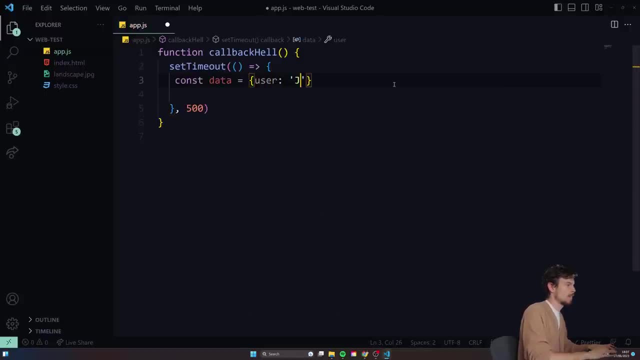 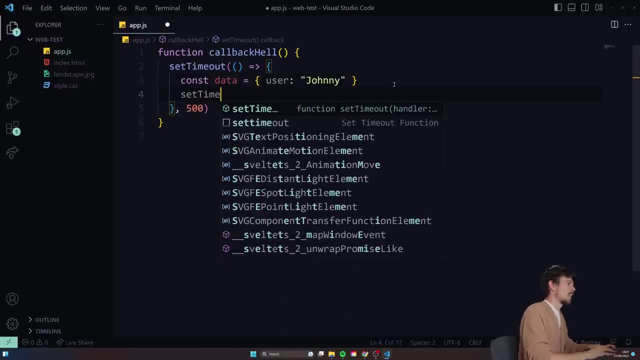 equals. let's say we have an object with a user of Johnny Boy And hit save, Cool, All right. So after this I need to. let's say I want to run another set timeout here. Let's say I want to. 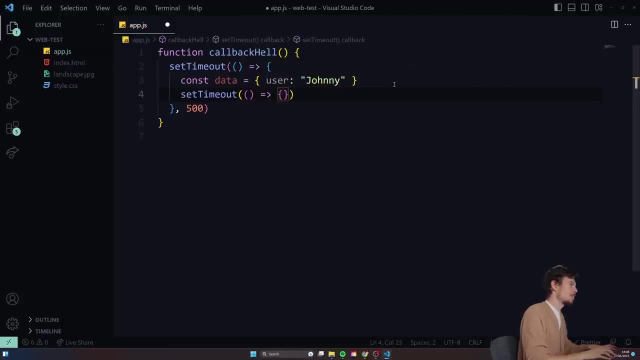 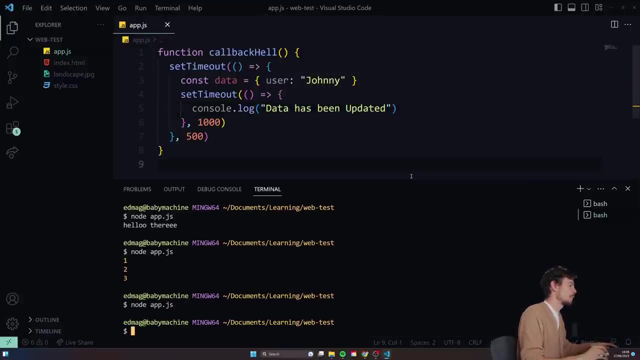 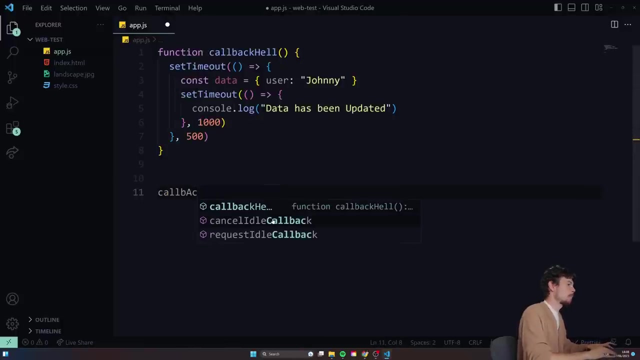 take this data and modify it and push it back, maybe to the database or something. So maybe this takes another thousand seconds. So here I can say data has been updated, All right, So if we run this, we wait a little bit. Oh, I never ran this function, Sorry. Callback Hell. 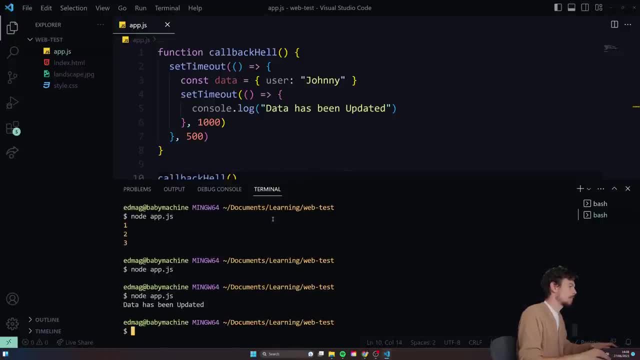 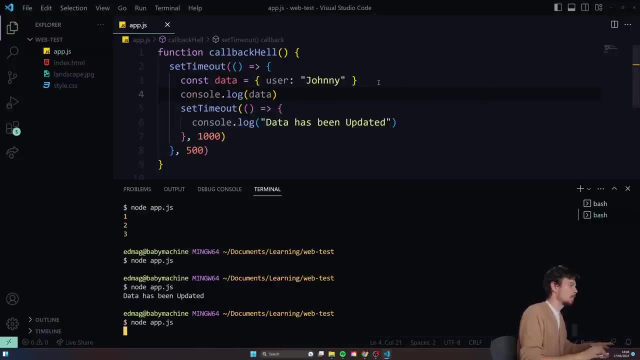 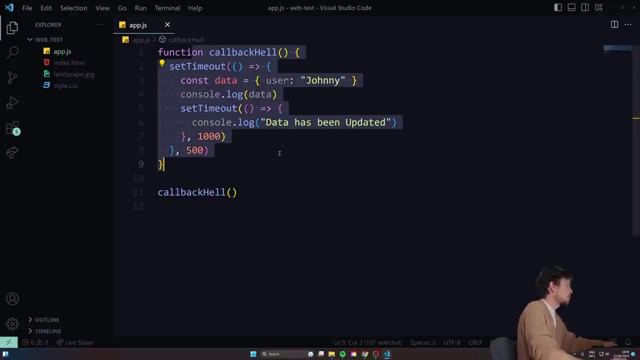 Let's execute this. Run. Data has been updated- Cool. Actually, I did not even console log out the data here. Boof User Johnny. Data has been updated, Cool. So essentially, the idea here is that it's an effective way to ensure delayed execution. 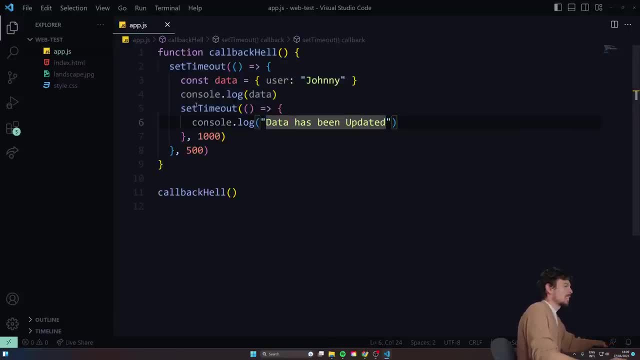 Functions until the other one completes and returns with some data. But the way they look usually is quite nasty, So we want to avoid it, So I wouldn't even bother with it. So what are promises? Promises are just the completion of an asynchronous function. Okay, We're expecting a. 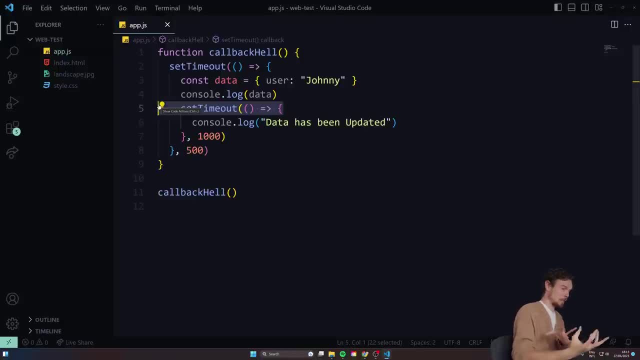 result back in the future, or maybe an error back in the future, And based on that error or success, we want to do something with it, Like display it on the screen or order fetch more data. All right, So it essentially accomplishes the same basic goal as the callback. 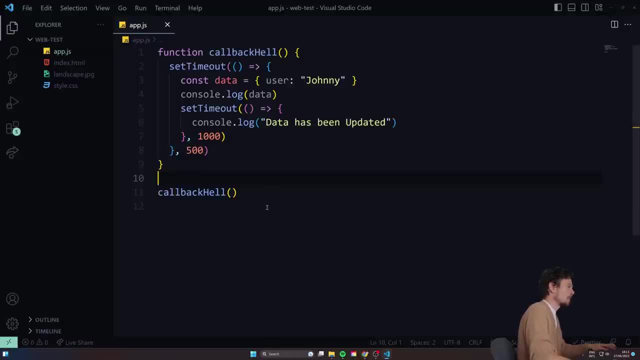 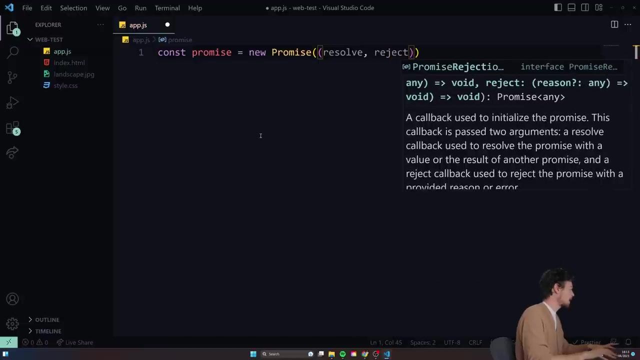 functions, but with many more features and a more readable syntax. So let me show you an example of how you can create the promise. So you just say const promise and you can set that equal to a new promise, like that- And this is going to take in a resolve and a reject parameter like that. 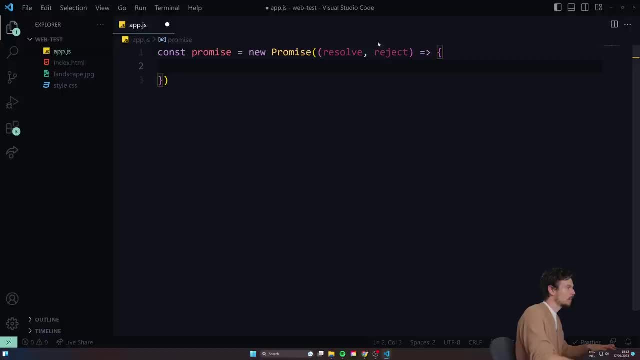 All right, And in here what we do is we either resolve it or reject it. So I can say: resolve, We did it, Maybe like that, Cool, And now I can take this promise like that and attach a dot, catch finally, or then on it. So when I add the dot, then here essentially I get back. 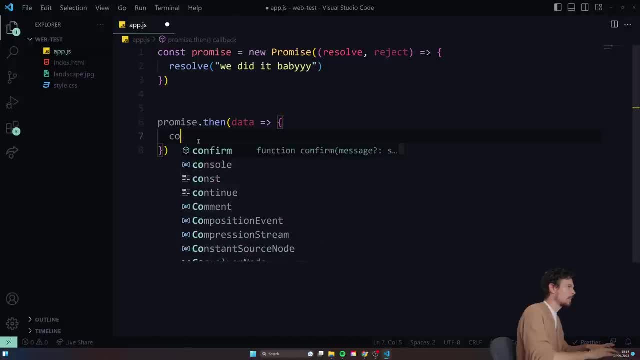 the resolved Data from it. So if I console, log data and save and we run this, we did it, baby, All right, So it got resolved. Now we can also reject it. Oh shit, Server is down. boys, Hit, save, We run this. 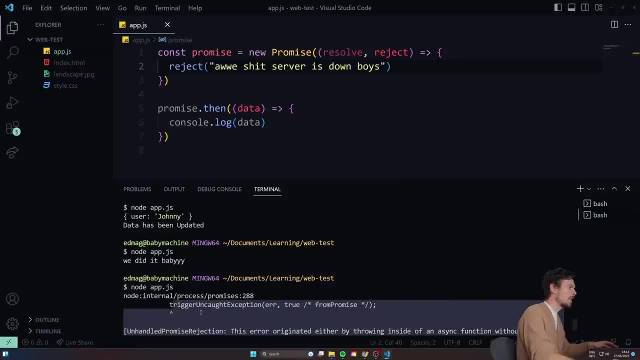 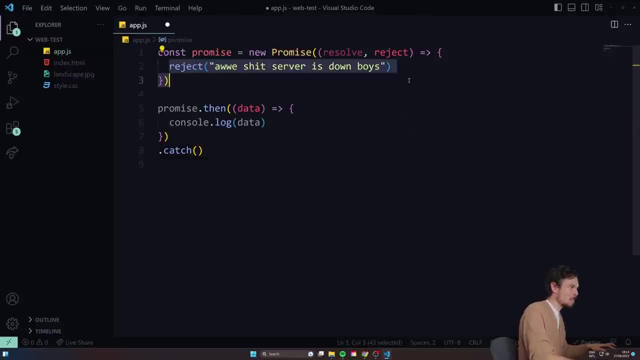 and we get an error, All right. So you're not going to get anything here unless you also add a dot catch. So a dot catch is basically: I got to catch any problems in your promise. So if there was a downtime, you maybe. 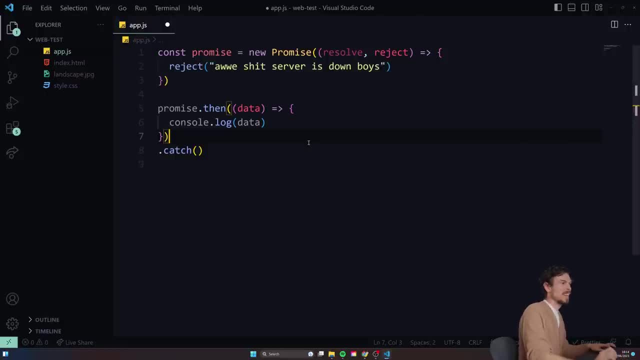 don't have the credentials to view the website. it might throw you back a wee error, right? You're not authorized to view this content on this page, or you might not be a member. So in this catch, you can get any exceptions from this reject. So, if I console, log out. 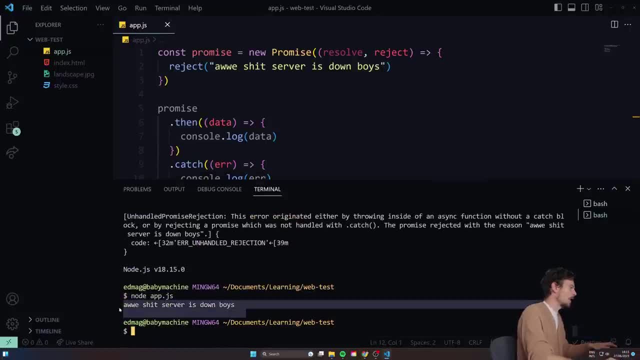 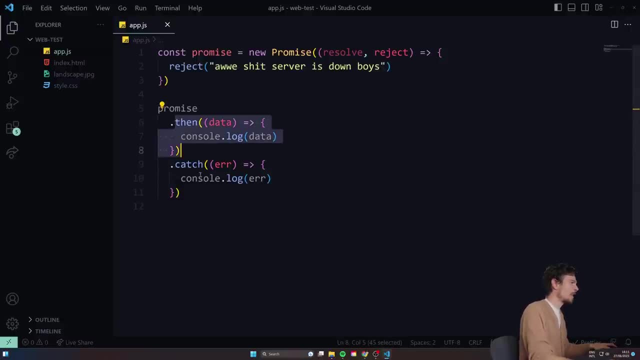 this error you're going to commonly see that. Look at that. Oh shit, Server is down, All right. So if the promise does not get resolved in any way, it's going to skip all of this dot then, because this dot then can kept being chained on and on and just is going to skip directly to the 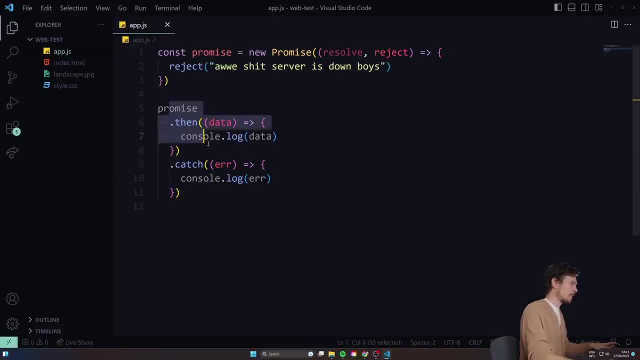 sketch: All right, Boof Error, And what I mean is that we can keep adding dot. thens, Let's resolve this. in this case, I'm going to say we got the, let's just make an object. Okay, And we have a user called Blanca. I'm playing. 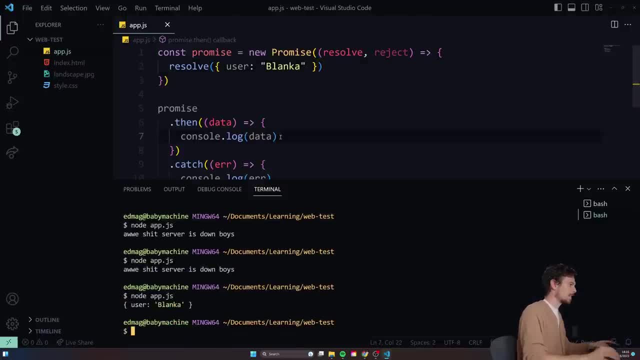 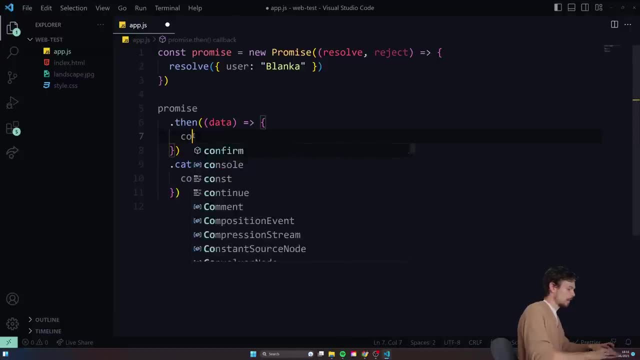 Street Fighter. It's fantastic, Okay. So if we run this, okay, we got Blanca there, Cool. But what I can do here is const data. Oh, let me call this user and set that equal to, maybe data, or I can just return data like that. And if I return data here, 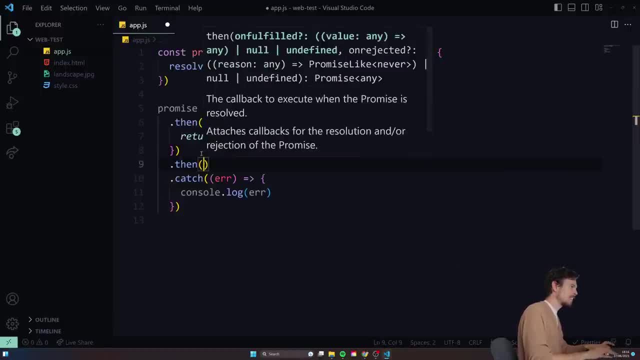 what that means is I can add another dot then on it and I'll have the actual user here like that: Oops, I messed up this dot. then It should have two parentheses, like that: User. All right, Console log user. So. 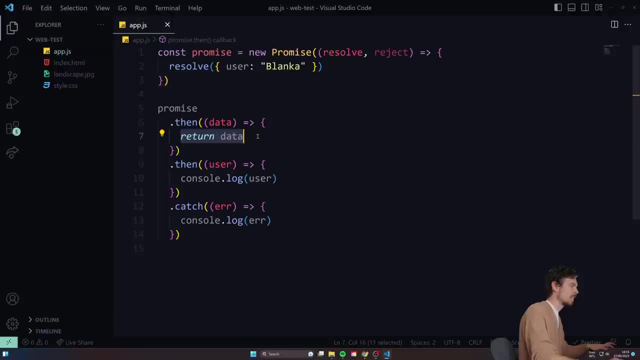 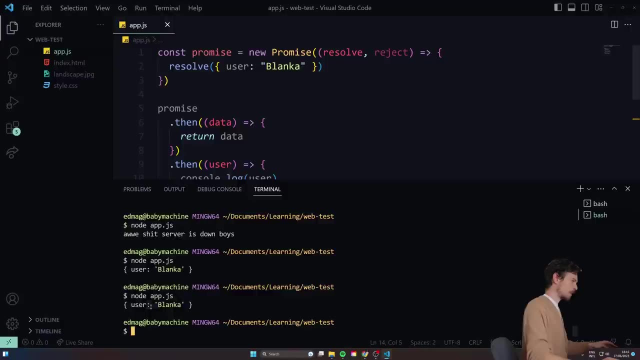 anything that should return here and the dot then is going to automatically go down to the other dot then here, so we can use it. So run this and we get user Blanca as well, All right, Or if you're not returning, maybe you're returning another. 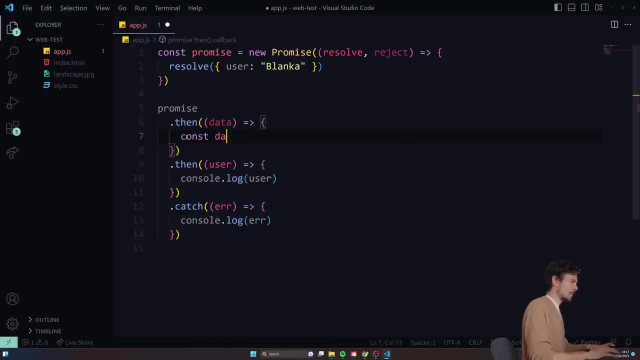 maybe we're just saving the user here. Data is sorry we can do. user is equal to data dot. I just called it data, right? You might want to return and maybe run another fetch here So we can go over to wwwgooglecom. So this return here now is going to be the actual data. 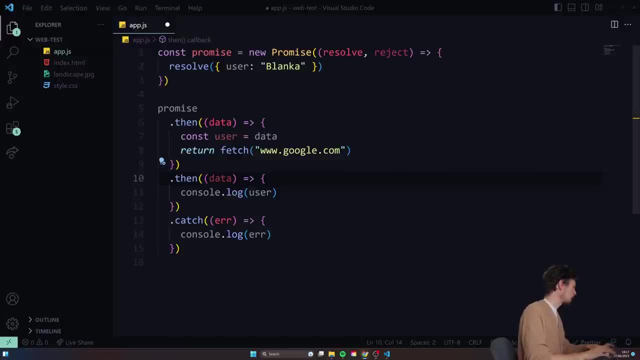 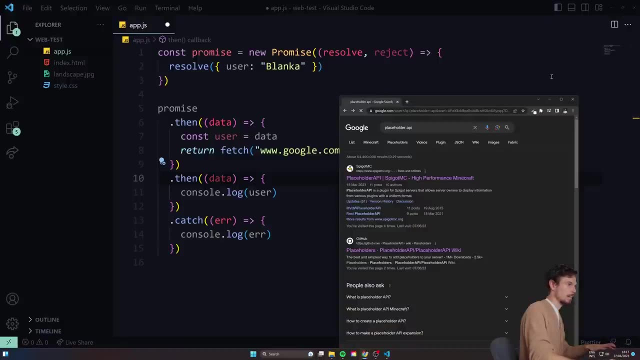 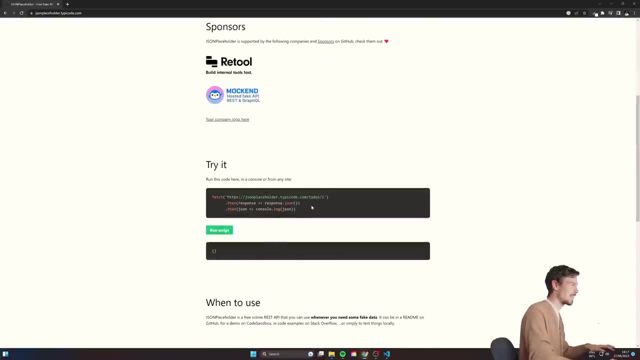 from whatever we're fetching from Google. Or let me go to placeholder API and actually fetch some real world data. Where is it? Let's go here. Where's the good old placeholder API to use? There we go, All right. So if I pass this in, 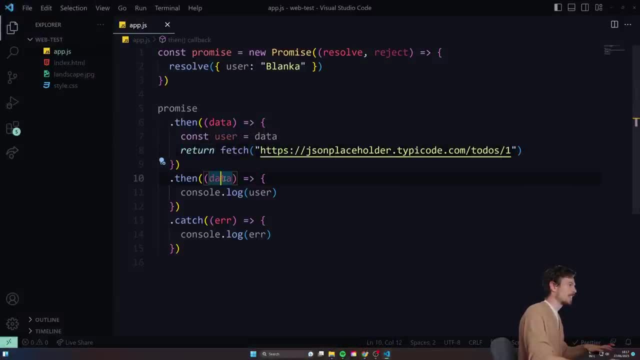 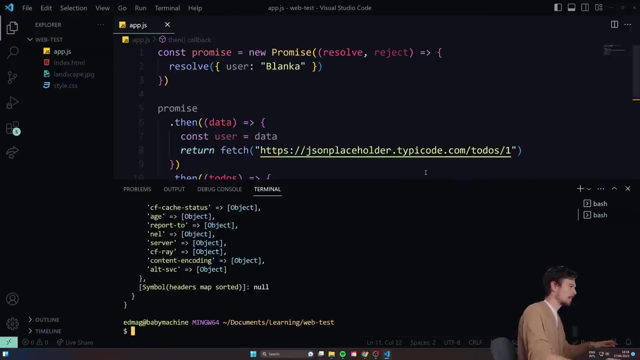 here in my return, then this data here is going to mean the actual to-dos from the placeholder API, So to-dos like that. So if I do a console log to-dos and run this, look at that. We're going to get our actual response. All right, So you can change. 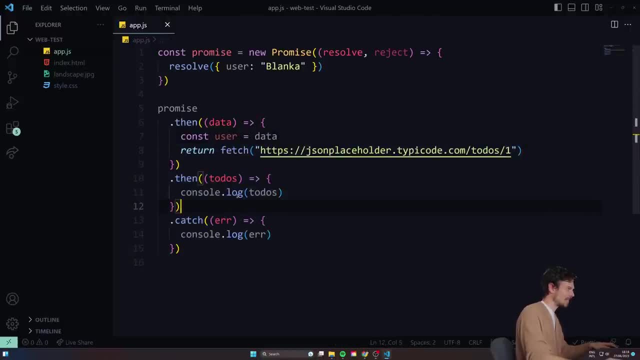 we're going to get our multiple dot thens, giving you a more simple syntax on how your code actually works. So let's go back to that first example with the set timeout and see how it would look So I can say: cons, promise, set a new promise like that Again. 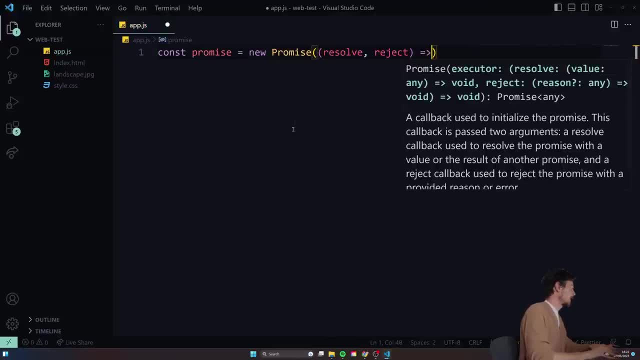 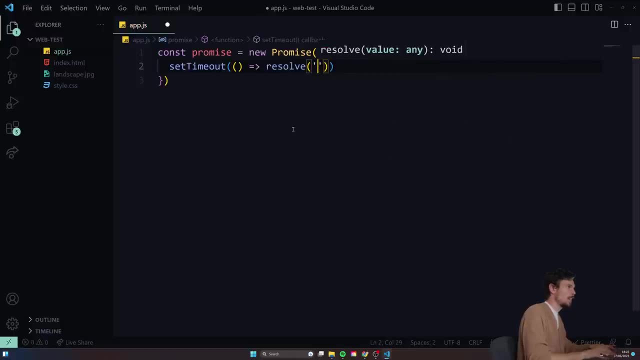 this is going to take in a resolve and a reject, Cool, And here I'm going to do a set timeout and let's say this is going to take maybe. hello, this is my data. This is my data from a. 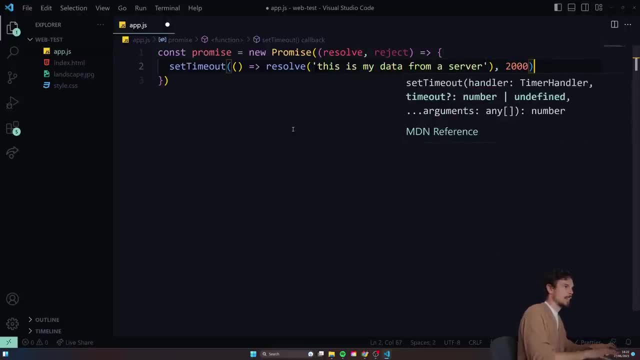 server. This is going to take, let's say, 2,000 seconds to resolve. okay, Milliseconds, Okay. So let's see how it works now. So I can just say promise and add a dot then to it. 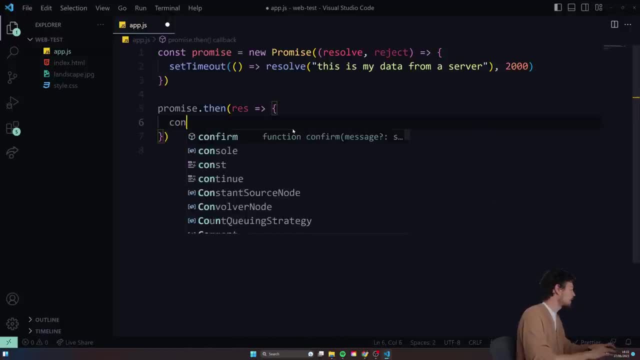 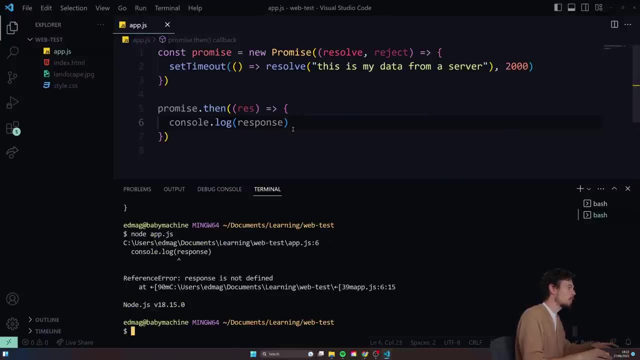 and then I get my response right here. I can just run an arrow function and say console log response And hit save. And now if I run this one, two and boom, Oop Res, not response. There we go, Run this again. 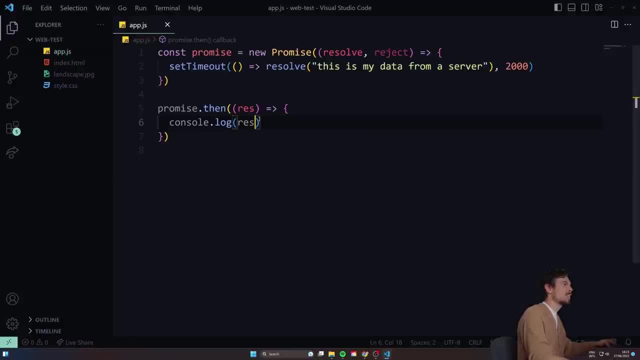 One, two and there we go, All right. So it makes it a bit more simple and readable on how, like, what is actually going on here. Now again, in most cases you're not going to create promises just for yourself out of the blue. You're probably going to use something. 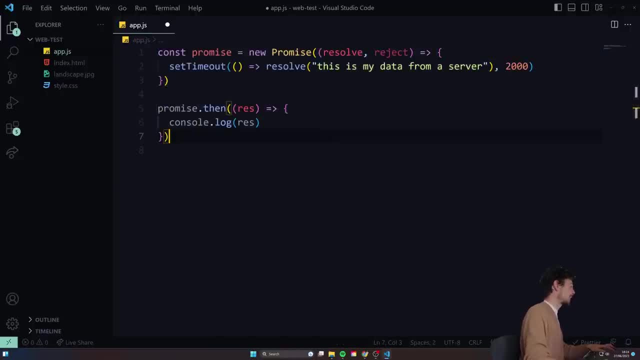 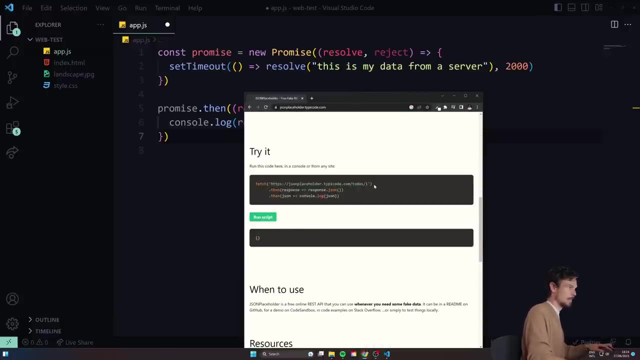 like the fetch API, which is going to return you a promise by itself. So if again I get the placeholder API, placeholder API, let's just get this and pop it in here. So if I do fetch here like that, that's automatically going to return me a promise, as you can see. 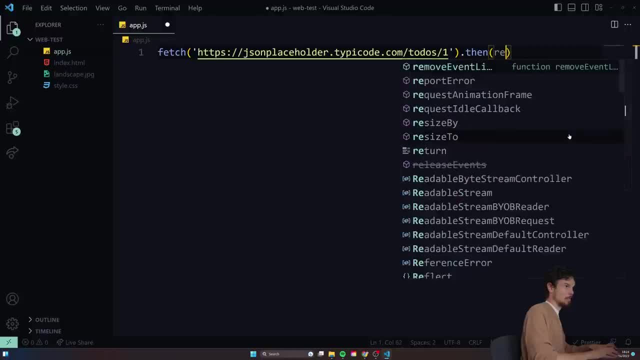 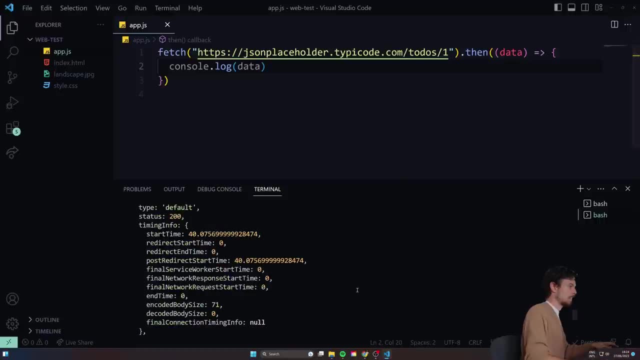 So I can do dot then again, which is going to give me the actual data, if everything goes through. fine. So console log data And we can run this, And there we go. There it is. We're going to probably have to do data. We can just return. 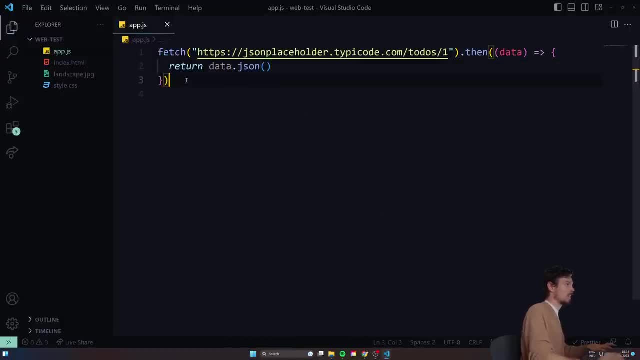 datajson. And again, if I do a return here that's going to be chained to the other dot, then All right. So here I'm actually going to have the JSON version of that data. So JSON data, So console log, JSON data, Run that and there it is. But what we can also do is attach a dot. 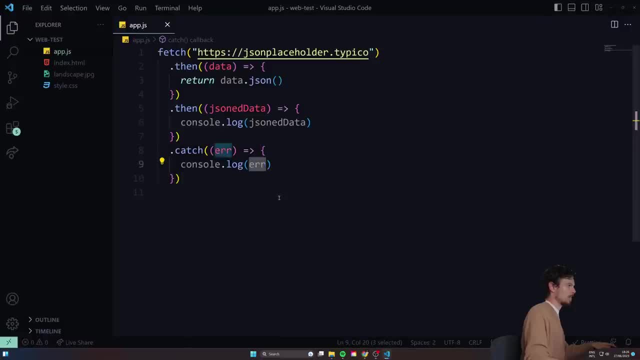 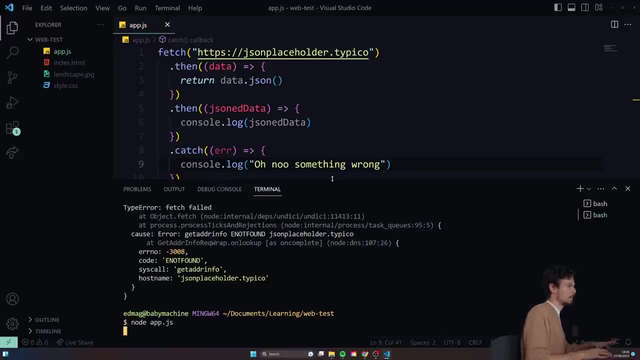 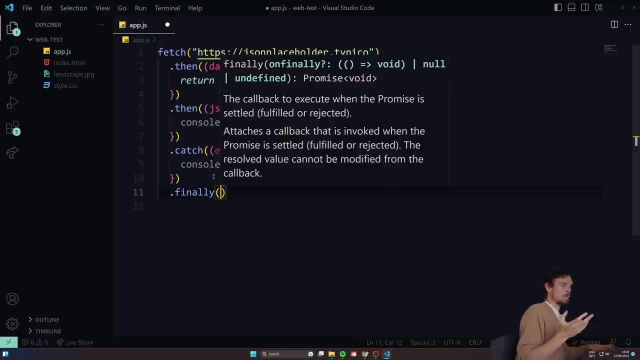 catch on it. So maybe the URL is not correct. So we can catch any errors here and say, oh no, something went wrong. If I run this, we got, oh no, something went wrong. And then you can also see there's a finally here And this is going to run, whether the 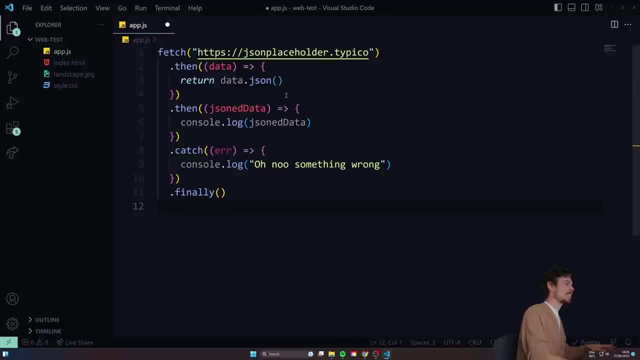 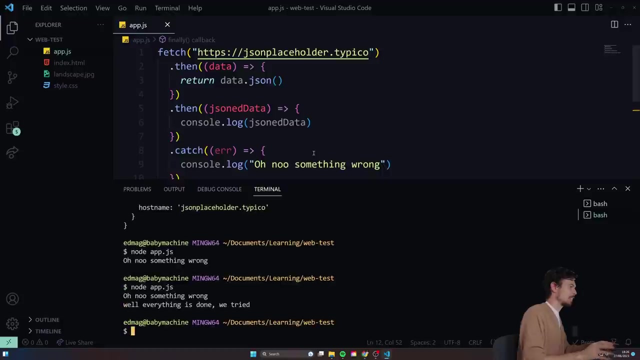 promise is rejected or resolved, It doesn't matter, At the end it's going to run finally anyway. So here I can say something like: well, everything is done, We tried All right And hit save and run that again, And there we go. So this is really nice, But with the introduction of ES6,, 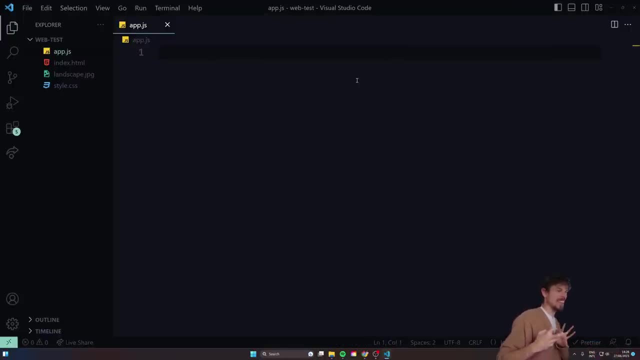 we have async and await, which essentially is just syntactical sugar over the promises to make it look synchronous and very easy and readable. And the way you make it is: you create a function and you add the async keyword in front of it. All right, So let's say we're getting the to-dos. 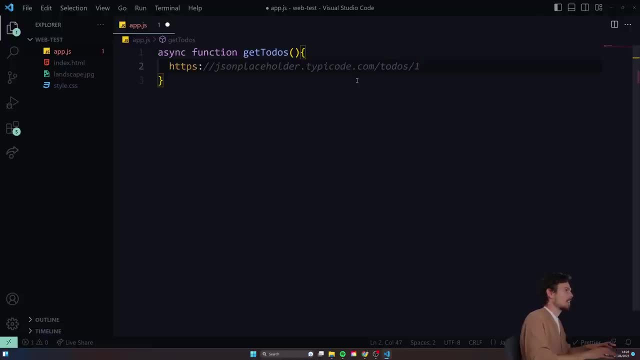 All right. So rather than doing how we used to do a fetch, you'd fetch the actual URL and then you'd attach all of these dot thens. So, instead of doing a fetch, you're going to attach the to-dos. So. 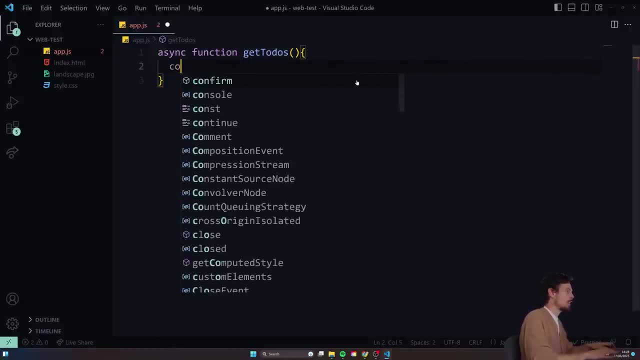 here. I'm going to attach the to-do, All right. So since this is working, I'm going to do a stash. So these dot dens on it. you just make a. let's just make a variable called response And we can use this await keyword. 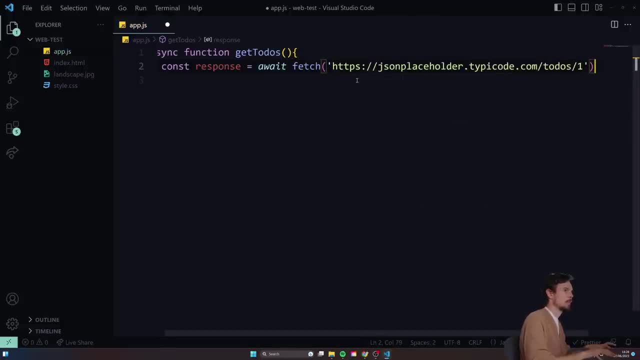 to await the result of this fetch call, all right, And that gets saved in here And that's it. So if I do a console log response and a console log, let's say two, all right, Just a random number, And then I can do a console log one, maybe on top of this. 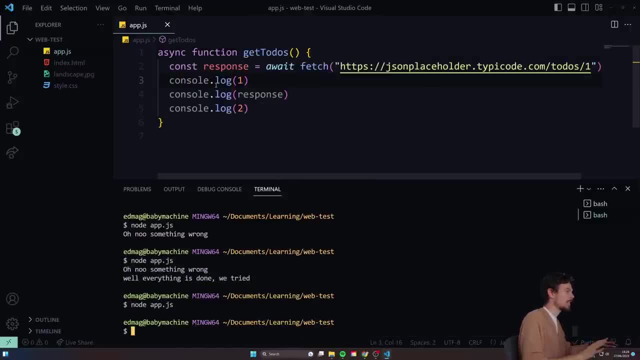 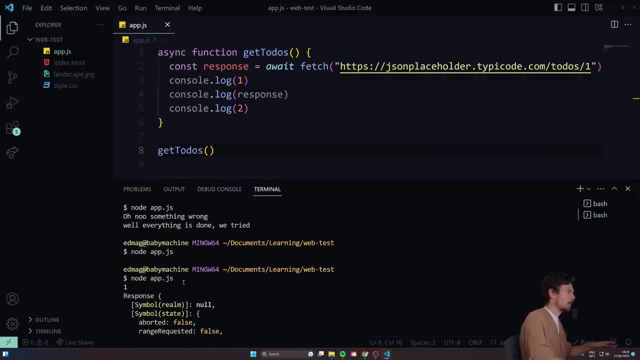 Console log one: Let's hit save and run this. Oh, I need to actually invoke this function. There we go And run this And if we have a look, we have one, we have the response and then we have two. 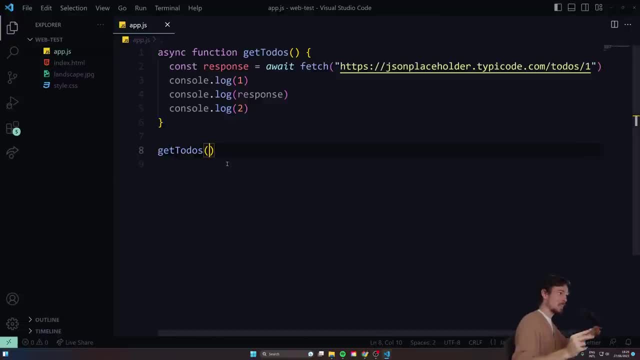 So it gives you the ability to have a synchronous code like synchronous looking syntax. I should say That's very easily readable and you know what the hell is going on. So here, if I wanna make this a JSON again, I don't need the dot then to make it JSON. 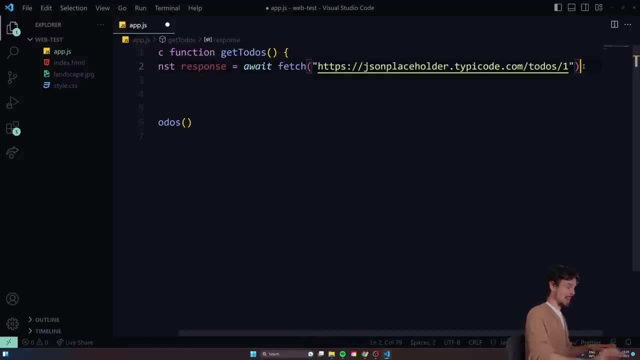 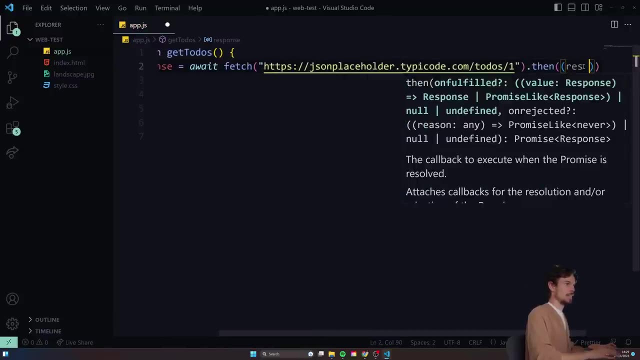 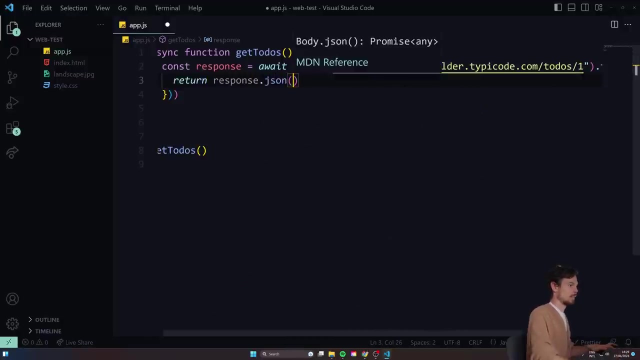 though you can, I can still go here even though I'm using await. I can still chain a dot then on it like that and say: well, just take this response and return me a response, dot JSON, Or what did I call this? 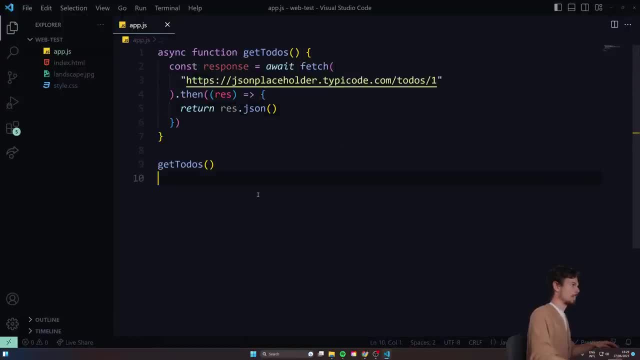 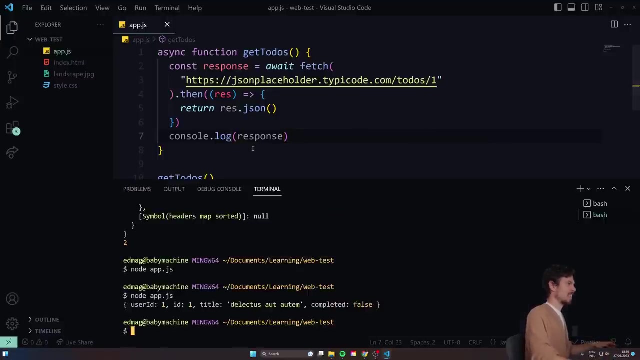 Res dot JSON. Res dot JSON. all right, So if I run this again, whoops, And I'll just go out here actually and say console log response like that. All right, so I still have the ability to do this, but there's no point to it when I can just get rid of it. 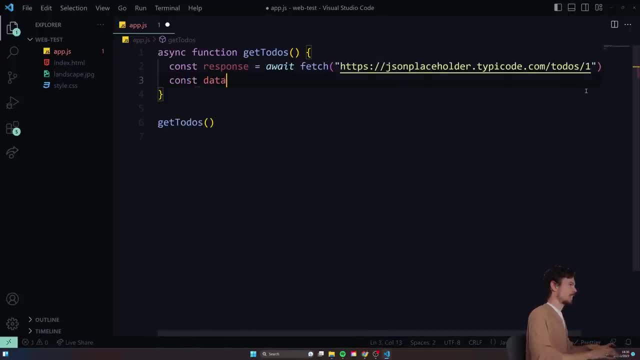 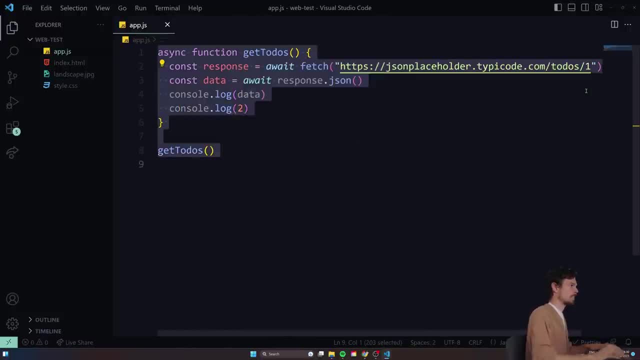 So then I can do console log, data, console log, whatever the rest of my code is down here. If I run this two, we get the data and we get two. Now be aware that in many new environments, like new versions of node and some browsers, 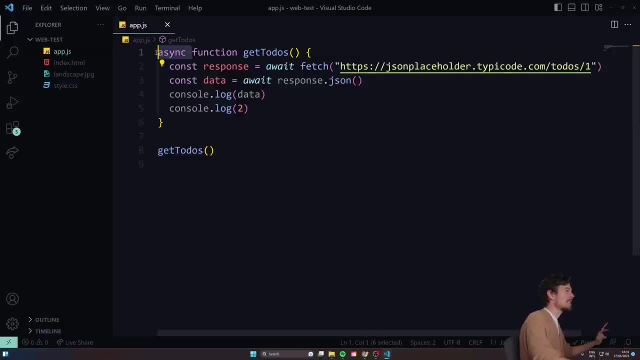 have the ability to not even need to create async and just have top level awaits. So essentially you could get rid of async there and add it to a function and just do await in the top execution context like that. All right, Which makes it even nicer, thankfully. So now you just 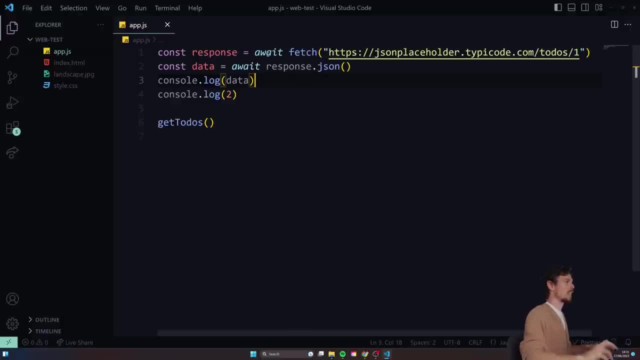 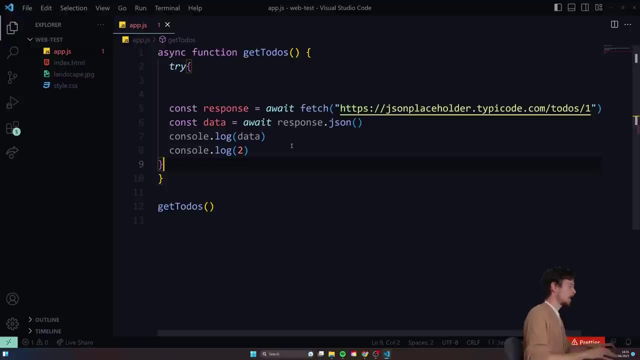 know, if you see an await, okay, that's some code that's going to run asynchronously And in terms of error handling, what you can do is wrap up your asynchronous code in a try- catch block, So you could go and do a try and let's pop that in like that, And then here I can say: catch any errors. 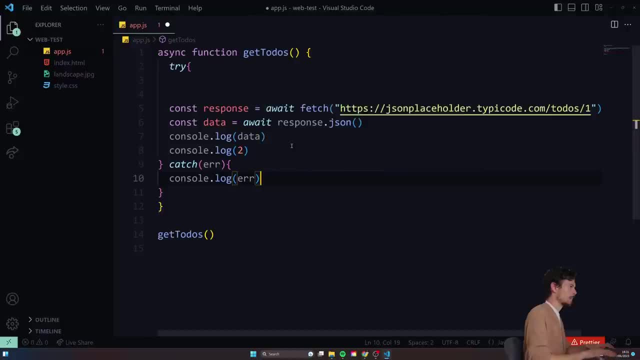 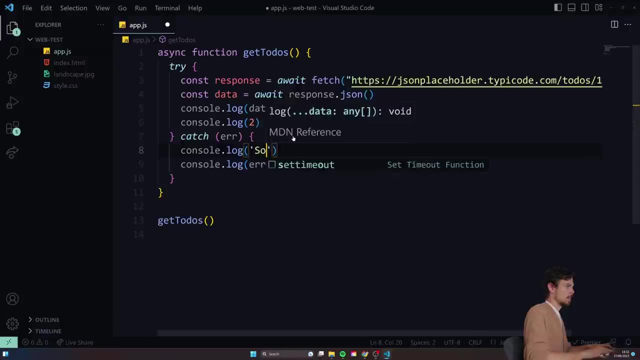 like that And I can say console log error and hit save All right. So now, if let me also do a message here, something went wrong, dot, dot, dot, Cool. So let's say this is not returning something correctly and run this again.